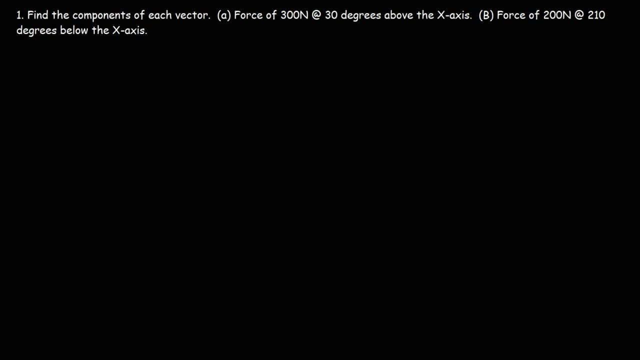 In this video we're going to talk about how to find the components of a vector. So in part A we have a force vector with magnitude of 300 newtons and the direction is 30 degrees above the x-axis. So let's begin by drawing a picture. 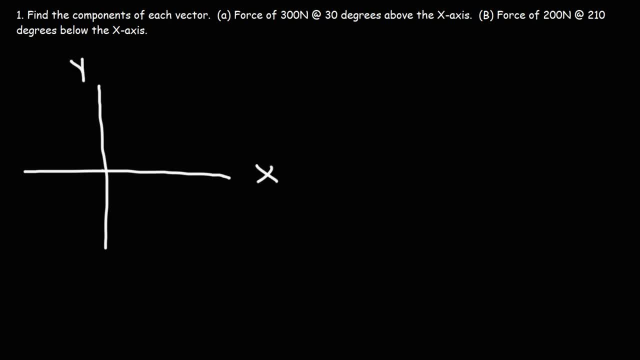 So here we have the x-axis and the y-axis, And here is our force vector at an angle of 30 degrees, and we have a magnitude of 300 newtons. So what we're going to do is we're going to turn this into a triangle. Here is the x component and here is the y component. 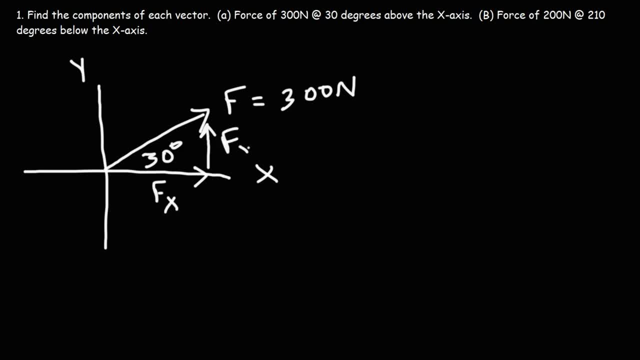 So this is the x component of the vector fx, and fy is the y component of the vector. To find the x component, you could simply use this formula: It's f cosine theta f is 300, and then we're going to multiply that by cosine of 30 degrees. 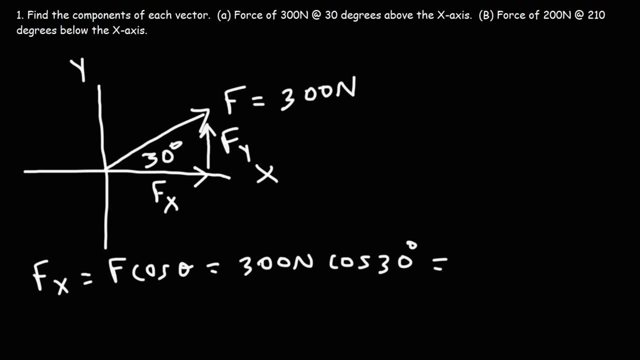 Cosine 30 is the square root of 3 over 2, which is 0.866.. If you multiply that by 300, you're going to get 259.8 newtons. So that is the x component of this force vector. Now let's find a y component. The formula that we need for that is f sine theta. 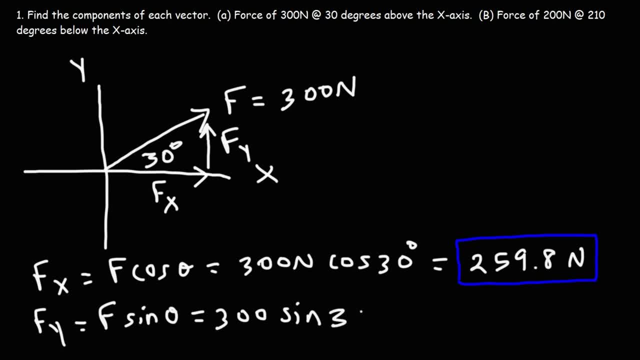 So this is going to be 300 times sine of 30 degrees. sine 30 is 1 half. Half of 300 is 150.. So this is going to be the answer. Now we can represent The force vector like this, using the I and J unit vectors. 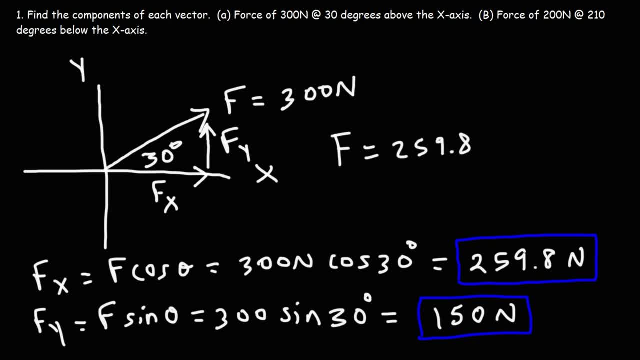 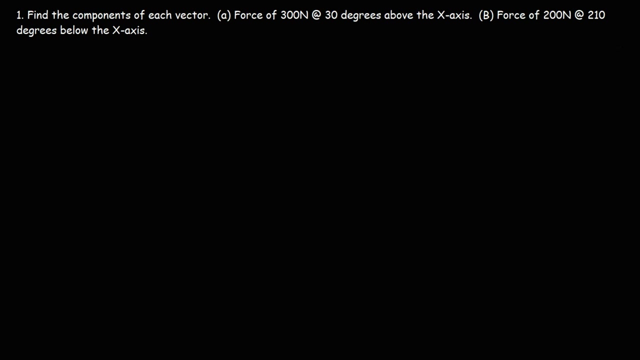 So this is gonna be 259.8 times the unit vector I plus 150 times the unit vector J. So that's how you can represent the force vector in component form. Now let's move on to part B. So let's begin with a picture. 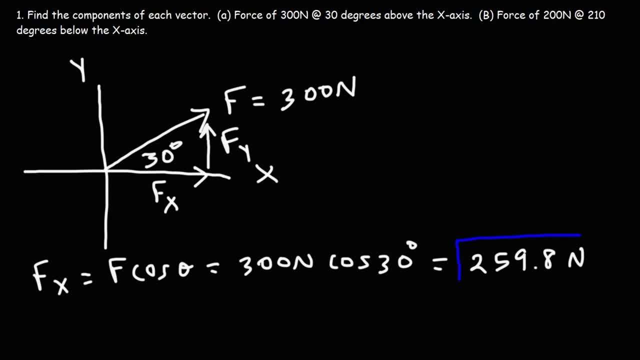 So that is the x component of this force vector. Now let's find the y component. The formula that we need for that is f sine theta. So this is going to be 300 times sine of 30 degrees. Sine 30 is 1 half. 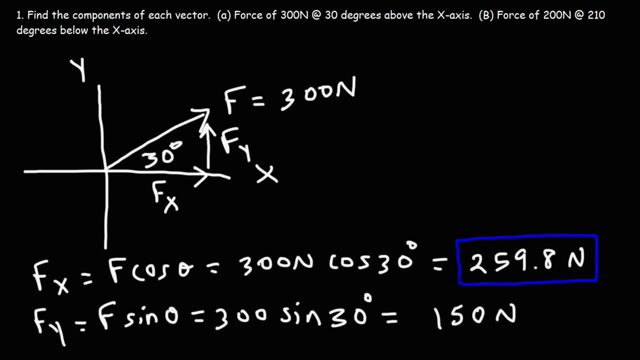 Half of 300 is 150. So this is going to be the answer. Now we can represent the force vector like this, using the i and j unit vectors. So this is going to be 259.8 times the unit vector i, plus 150 times the unit vector j. 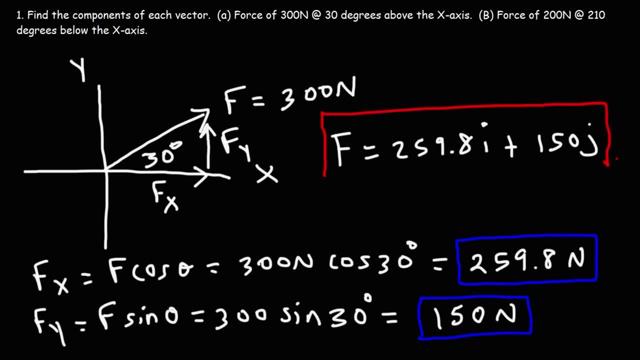 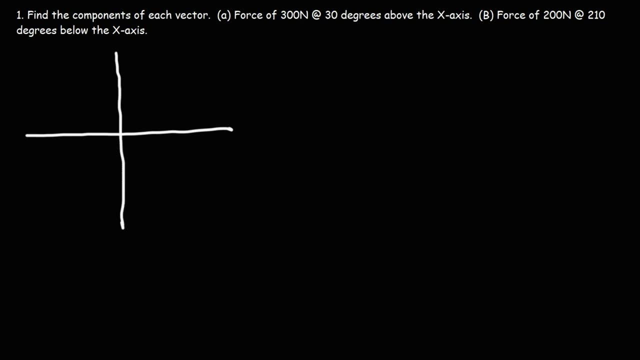 So that's how you can represent the force vector in component form. Now let's move on to part b. So let's begin with a picture. Now we have a force vector with a magnitude of 200 newtons and the direction is 210 degrees below the x-axis. 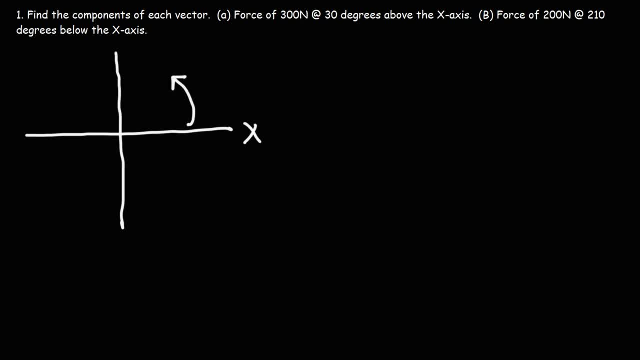 So, rather than going above the x-axis in the counterclockwise direction, we're going to go below the x-axis in the clockwise direction. So this is going to be 90 degrees, this is 180, and then 210.. 210 is 30 degrees more than 180.. 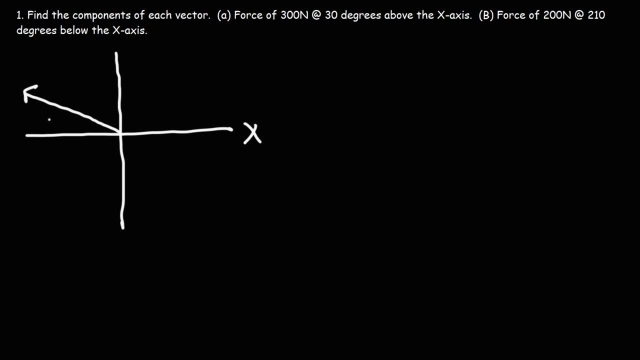 So our force vector is going to be over here and it's going to be 30 degrees above the negative x-axis And it has a magnitude of 200 newtons. So what I'm going to do is I'm going to redraw it like this: 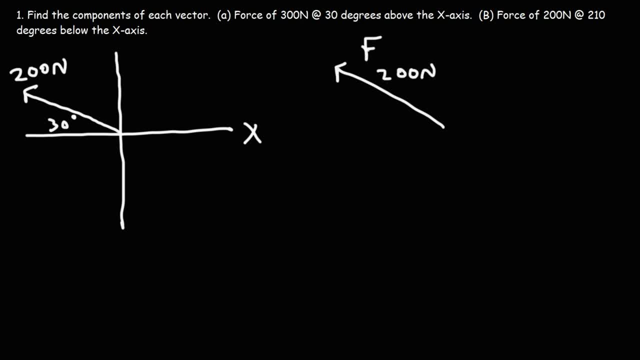 So that's f, this is the x-component and this is the y-component, and we have a reference angle of 30 degrees. Now this angle here from the positive x-axis, that's 150.. If you're going to use the reference angle of 30,, 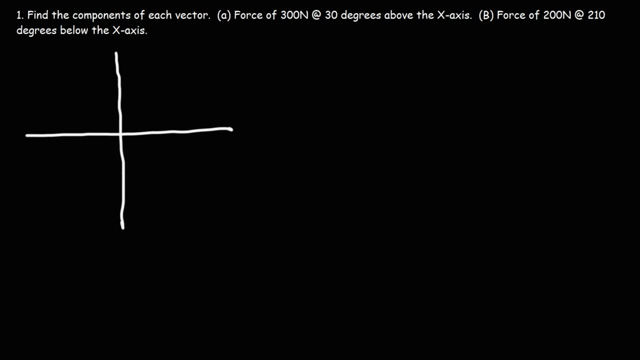 Now we have a force vector with a magnitude of 200 newtons and the direction is 210 degrees below the x-axis. So rather than going above the x-axis in the counterclockwise direction, we're gonna go below the x-axis. 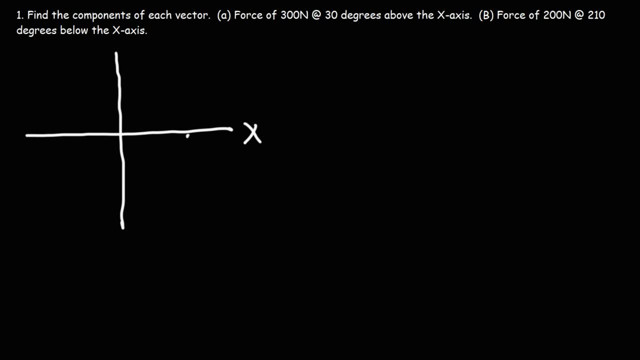 in the clockwise direction. So this is gonna be 90 degrees, this is 180, and then 200, 210.. 210 is 30 degrees more than 180. So our force vector is gonna be over here and it's gonna be 30 degrees above the negative x-axis. 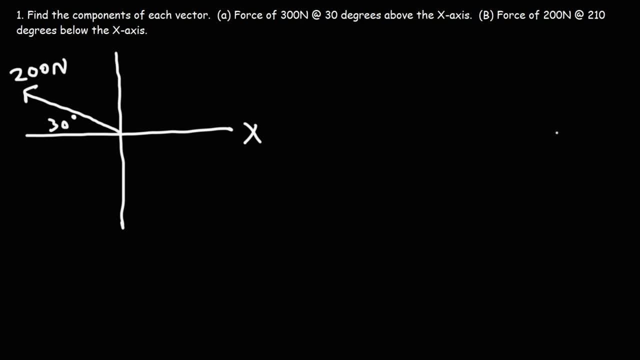 And it has a magnitude of 200 newtons. So what I'm gonna do is I'm gonna redraw it like this. So that's F, This is the x component, and this is the y component, And we have a reference angle of 30 degrees. 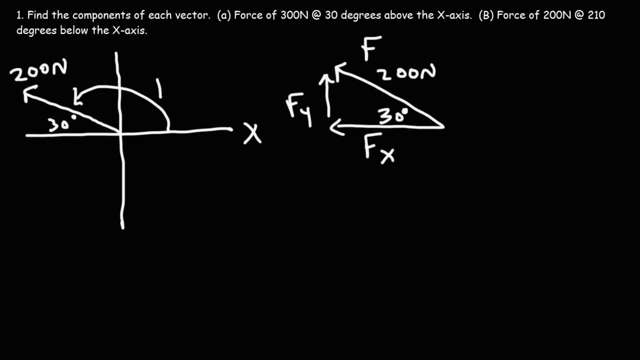 Now this angle here from the positive x-axis, that's 150.. If you're going to use the reference angle of 30, you need to add the appropriate signs, For instance In quadrant two. by the way, this is quadrant one, quadrant two, quadrant three, quadrant four. 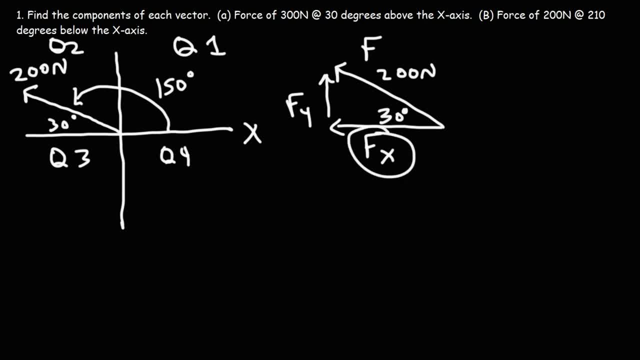 So in quadrant two, notice that x is going to be negative because it's to the left. Y is going up, so it's still going to be positive. If you were to use cosine 30, you would get a positive answer, But to make it correct you would have to add a negative sign. 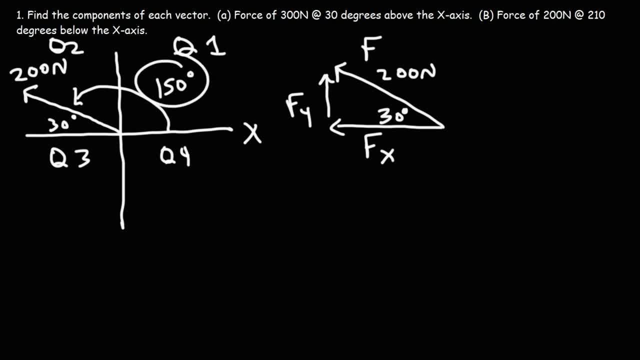 However, if you were to use the angle measured from the positive x-axis, if you were to put cosine 150, it would already include the negative sign. So you could use either one of these angles to get the right answer, But in the end you need to make sure that the sign is correct. 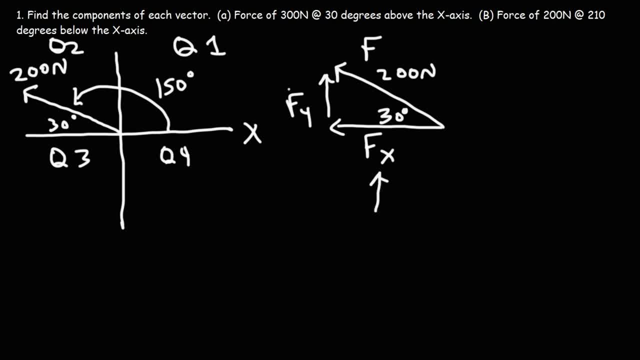 So because x is on the left side, it's going to be negative. Because y is going up, it's going to be positive. Now I'm going to use the angle measured. I'm going to use the angle measured from the positive x-axis in the counterclockwise direction. 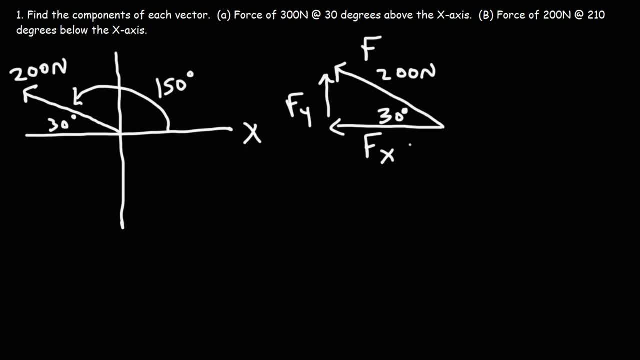 you need to add the appropriate signs, For instance in quadrant 2,. by the way, this is quadrant 1, quadrant 2, quadrant 3, quadrant 4.. So in quadrant 2, notice that x is going to be negative because it's to the left. 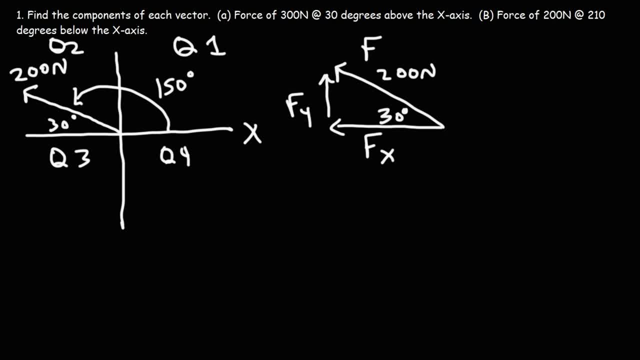 y is going up, so it's still going to be positive. If you were to use cosine 30, you would get a positive answer, But to make it correct you would need to add the appropriate signs. However, if you were to use the angle measured from the positive x-axis, 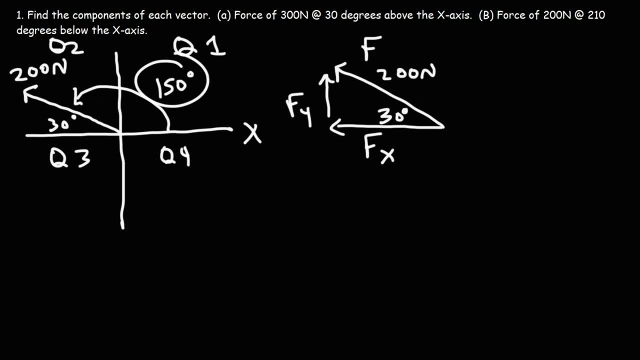 if you were to put cosine 150, it would already include the negative sign. So you could use either one of these angles to get the right answer, but in the end you need to make sure that the sign is correct. So because x is on the left side, it's going to be negative. 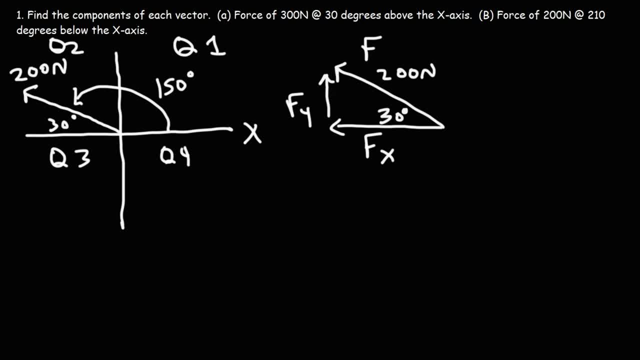 Because y is going up, it's going to be positive. Now I'm going to use the angle measured from the positive x-axis in the counterclockwise direction, And the reason for this is because it's automatically going to give you the appropriate sign. 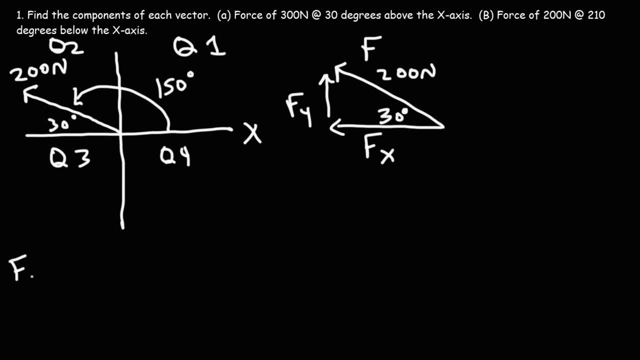 And it just makes things a lot easier. So let's get the x component. It's going to be f cosine theta, So that's going to be 200 times cosine 30. And we said that cosine 30 is root 3 over 2.. 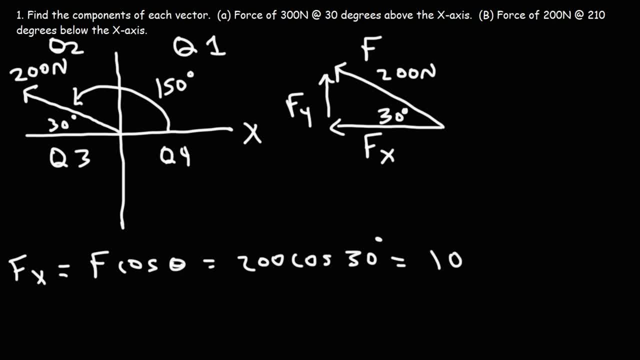 200 divided by 2 is 100. so the exact answer is going to be 100 square root 3. now for the y component. it's going to be f sine theta. you know what this should be? 2, i mean 150, and this is going to be negative 100 root 3. now for f sine theta, this is going to be 200. 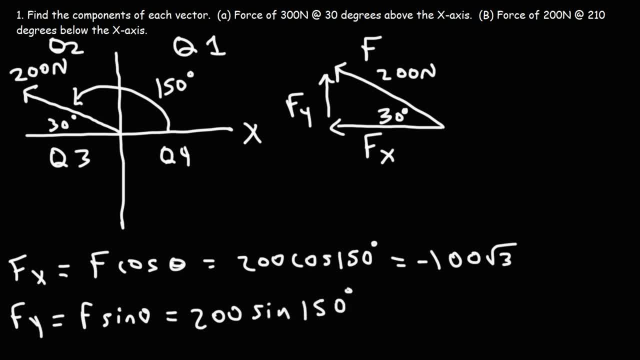 sine 150. if you plug this in your calculator, you're going to get 100 positive 100, and so this is going to be the x component and this is the y component. now let's write our answer in component form. now let's write our answer in component form. 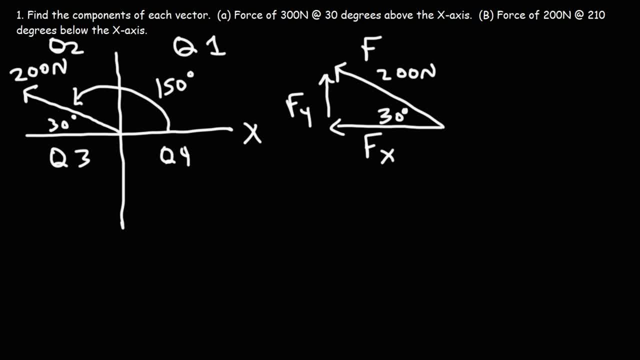 And the reason for this is because it's automatically going to give you the appropriate sign And it just makes things a lot easier. So let's get the x component. It's going to be f cosine theta, So that's going to be 200 times cosine 30.. 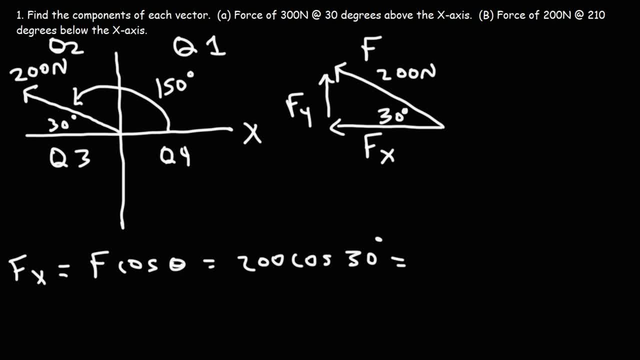 And we said that cosine 30 is root 3 over 2.. 200 divided by 2 is 100.. So the exact answer is 100.. So the exact answer is going to be 100 square root 3.. Now for the y component. it's going to be f sine theta. 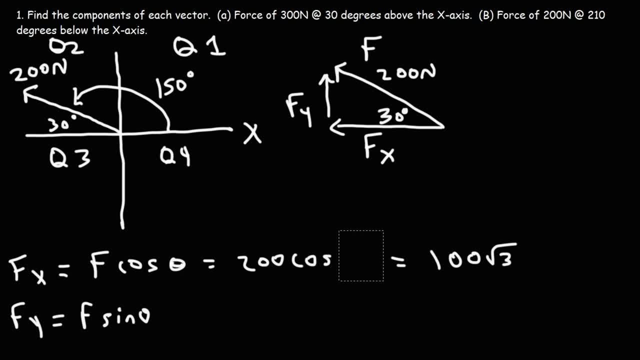 You know what? This should be 150.. And this is going to be negative 100 root 3.. Now for f sine theta. this is going to be 200 sine 150.. If you plug this in your calculator, you're going to get 100, positive 100. 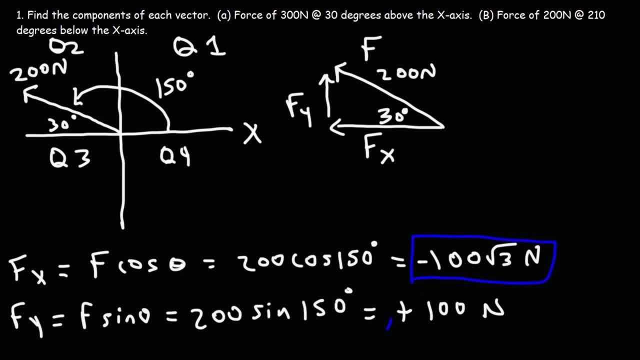 And so this is going to be the x component And this is the y component. Now let's write our answer in component form. So we could say that the force vector is negative: 100 square root 3.. You could put the unit newtons if you want. 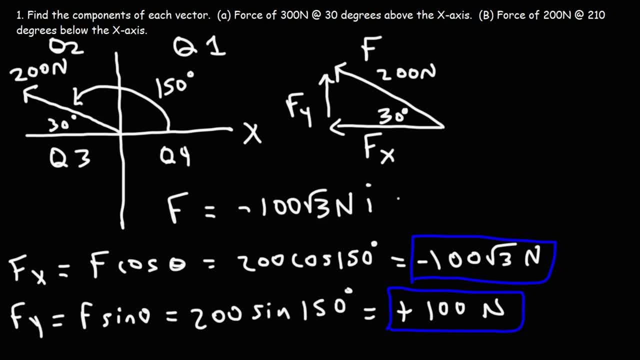 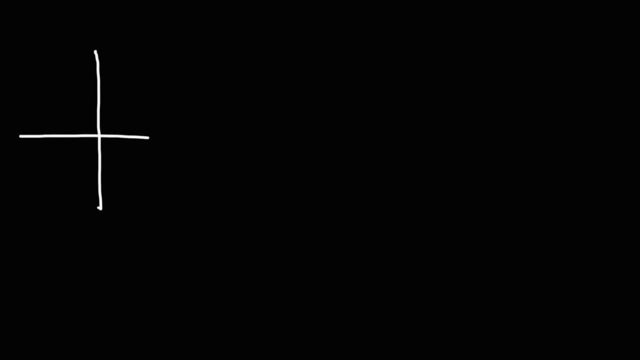 and then times the unit vector i plus 100 newtons and then the unit vector j. So that's it for part b. Now let's talk about the equations and why they are the way they are. So let's say: this is the force vector. 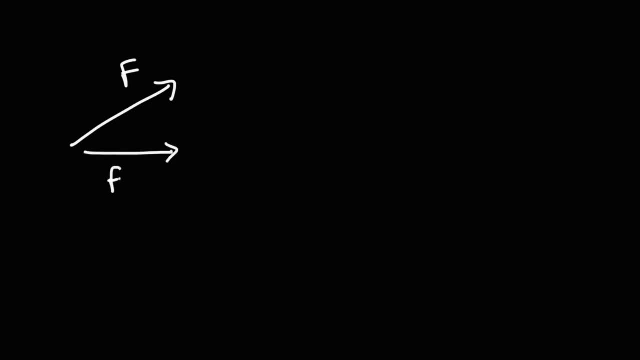 Let's say this is f, This is f of x and f sub y. And here's the angle theta. Now, in trig, perhaps you've heard of this expression, SOHCAHTOA. The SOH part means that sine is equal to the opposite side. 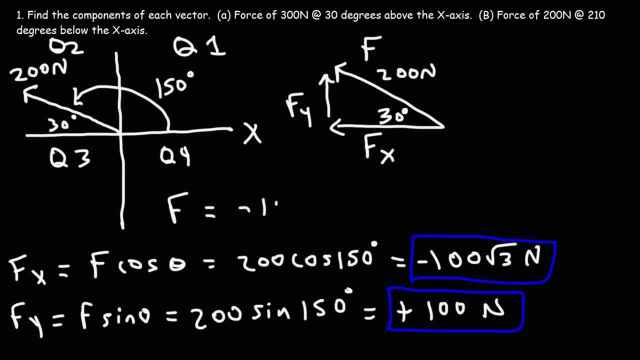 so we could say that the force vector is negative: 100 square root 3. you could put the unit newtons, if you want, and then times the unit vector i plus 100 newtons and then the unit vector j. so that's it for part b. 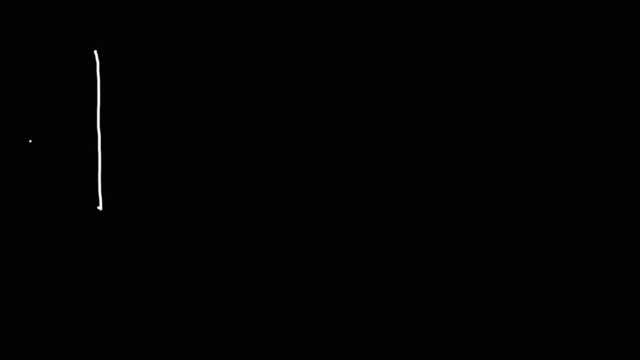 now let's talk about the equations and why they are the way they are. so let's say: this is f, this is f of x and f sub y. and here's the angle theta. now in trig, perhaps you've heard of this expression, sokotilla. the so part means that sine is equal to the opposite side over the hypotenuse. 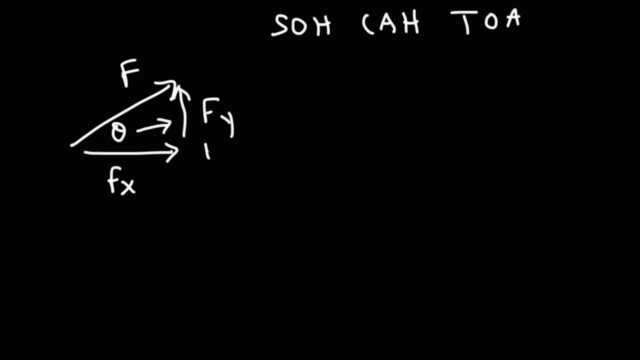 opposite to theta is F of Y, adjacent to theta is F of X and across the hypotenuse this forms a right triangle, I mean across the. the right angle, rather, is the hypotenuse, which is F. so using this part we have sine, theta is going to be equal to the opposite side, which is F of Y. 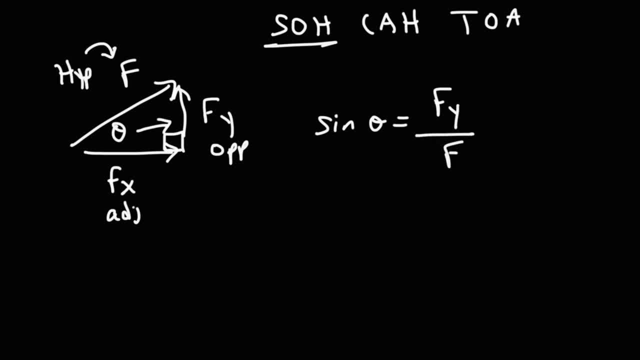 divided by the hypotenuse F. if you multiply both sides by F, you'll get this equation. the Y component is F sine theta. so it really comes from trig, particularly certain the circuit or equation. so it really comes from trig, particularly certain, the circuit or equation. so it really comes. 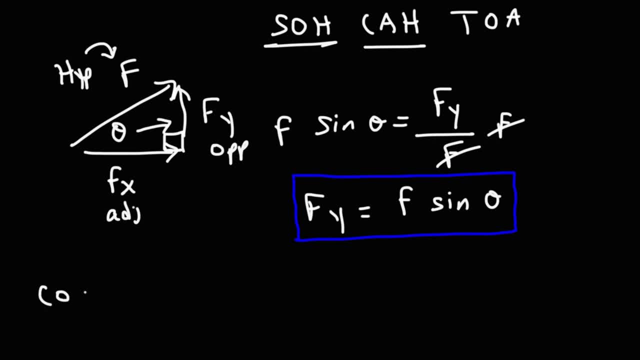 equation, so it really comes from trig, particularly certain. the circuit or equation, now the next one. equation, now, the next one equation, now the next one. cosine cosine theta is equal to the adjacent cosine. cosine theta is equal to the adjacent cosine. cosine theta is equal to the adjacent side, which is going to be F sub. 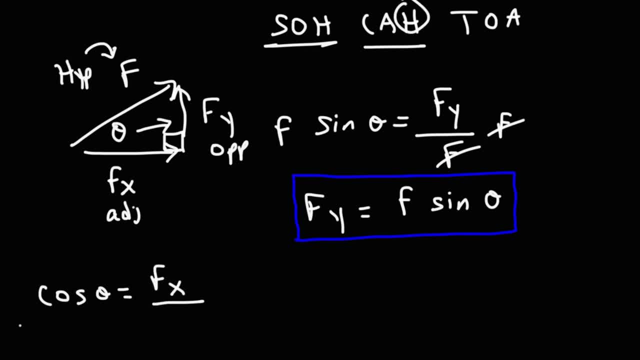 side which is going to be F, sub side which is going to be F, sub X over the hypotenuse which is F, and then if X over the hypotenuse which is F, and then if X over the hypotenuse which is F, and then, if we do the same thing, if we multiply, 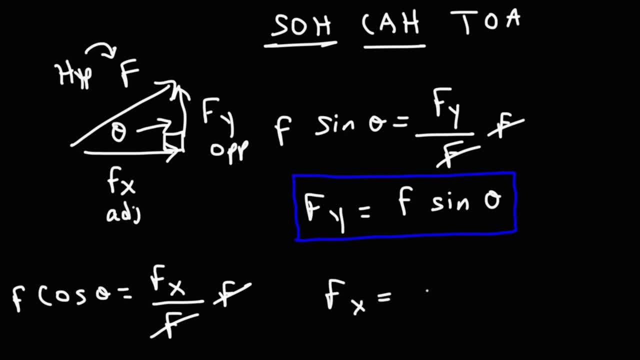 we do the same thing if we multiply. we do the same thing if we multiply both sides by F, we get that the X, both sides by F. we get that the X, both sides by F. we get that. the X, component of the force vector is simply component of the force vector is simply. 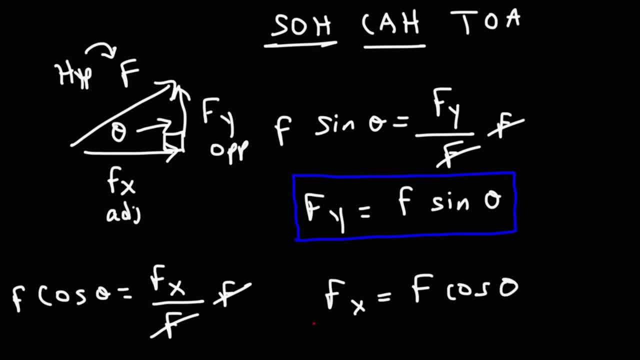 component of the force vector is simply F cosine theta. so that's where you can get F cosine theta. so that's where you can get F cosine theta. so that's where you can get these equations for those of you who these equations, for those of you who